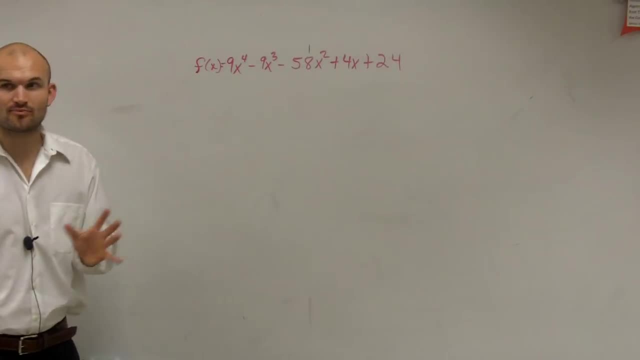 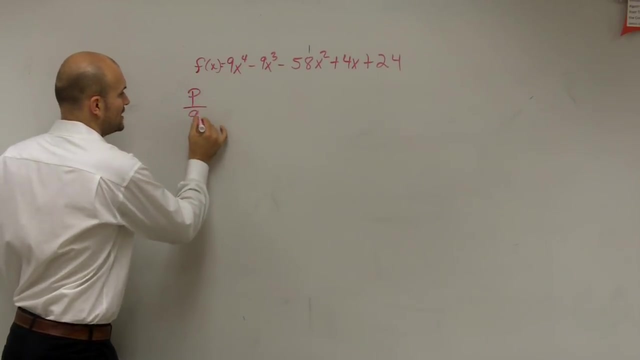 Then, once you guys get used to it and you understand what we're kind of doing, you can start breaking them down first of all, But remember to find all the possible rational zeros, that's going to be the factors of p over q. 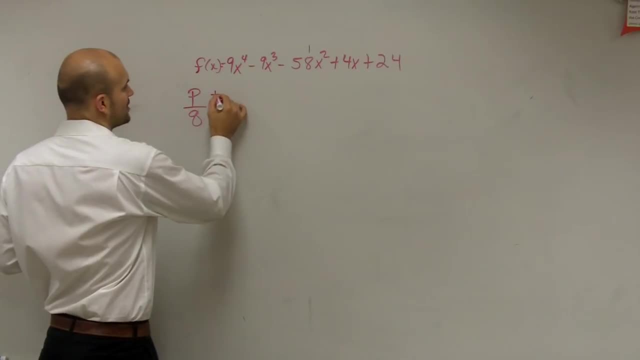 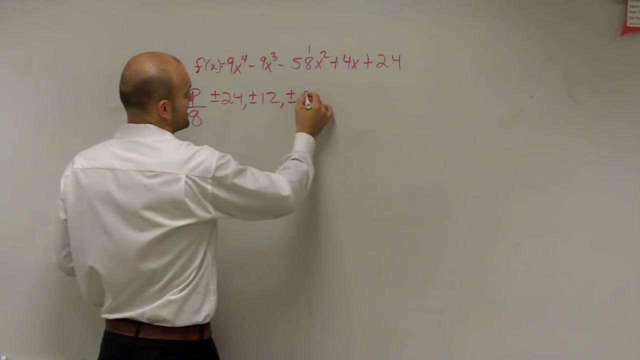 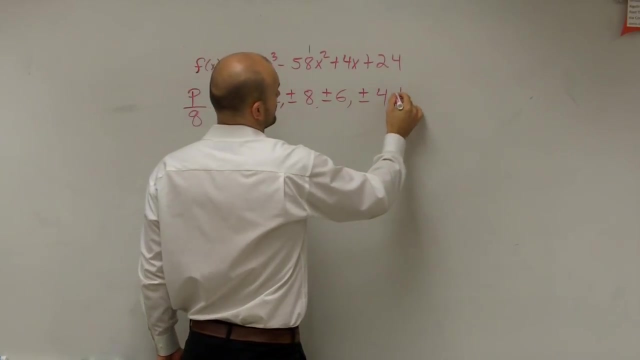 Alright. So let's look at all the factors of p over q. That's going to be plus or minus 24,. plus or minus 12.. That's going to be plus or minus 8,, plus or minus 6.. And plus or minus 4,. plus or minus 2,, plus or minus 1.. 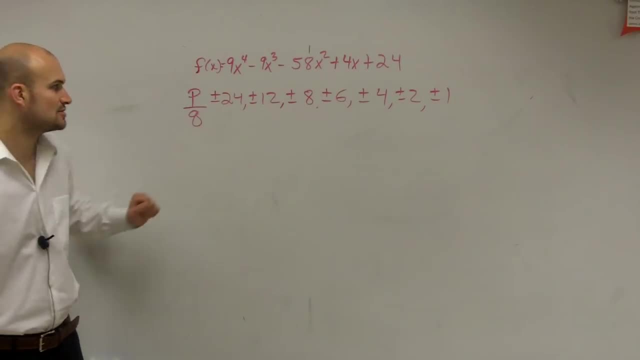 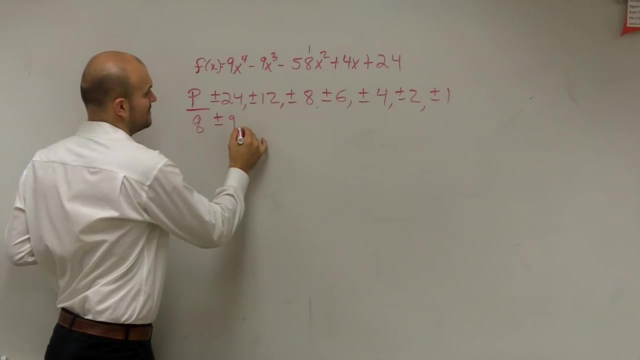 Correct. That's all the factors, Every single number that divides into 24.. Let's look at q, Our q, So that's going to be plus or minus 9.. Plus or minus 3. And plus or minus 1.. 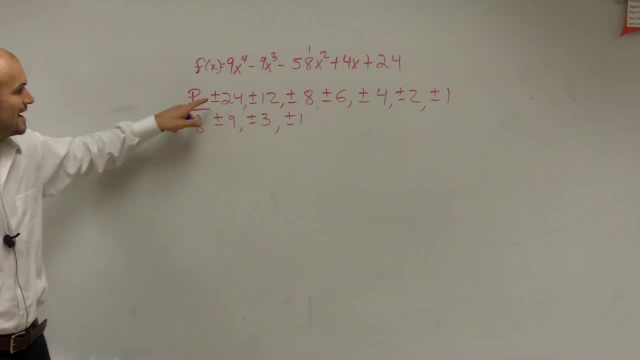 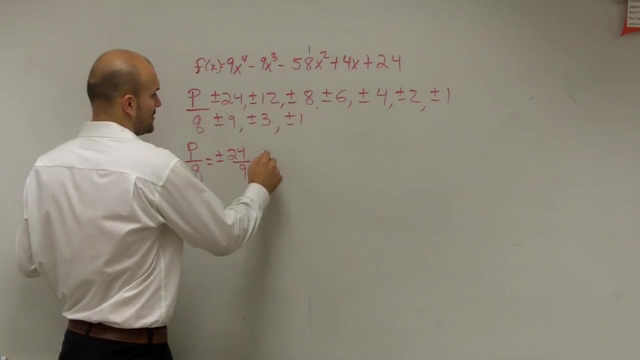 Alright. So what I need to do is I need to put every single one of these numerators over each one of the denominators. This is a big problem, right? This is going to be a lot of solutions. So p over q is plus or minus 24 over 9, comma. 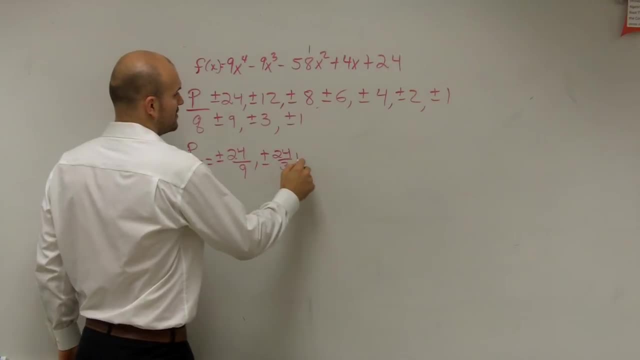 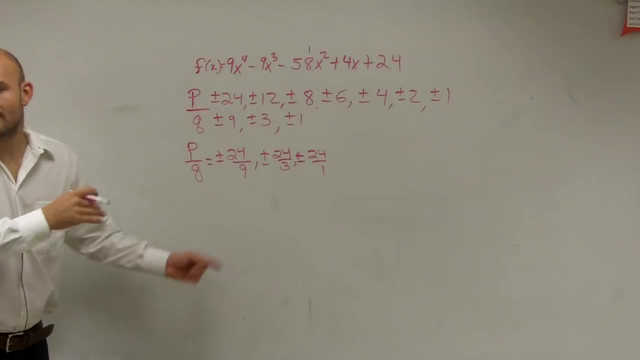 Plus or minus 24 over 3, comma. Plus or minus 24 over 1. right, right, I'm gonna, I'm gonna go and simplify them all. I'm just gonna write them all out and then you guys will see. oh, you don't need to write. 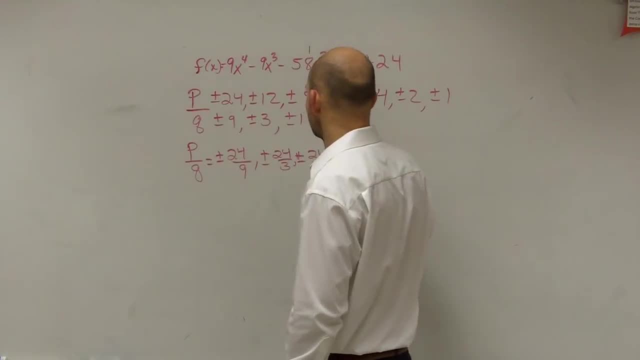 them all out. you can, can't, you know you can cut some out, if you don't. if once you see duplicates- because you don't need to write in duplicates- if you have extras, then you can eliminate them. so then I have plus or minus 12 over 9. 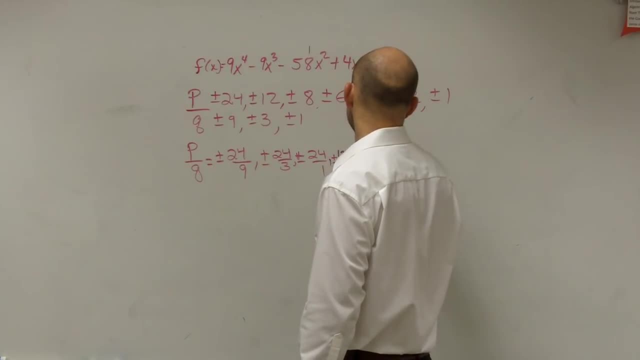 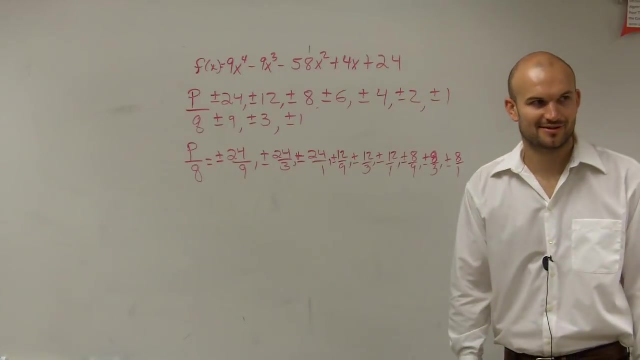 comma plus or minus 12 over 3 comma plus or minus 12. over 1 comma plus or minus 8 over 9 comma plus or minus 8, 8 over 3 comma plus or minus, 8 over 1. everybody kind of finally seeing my my trend that I'm doing here. this is a lot of problems. 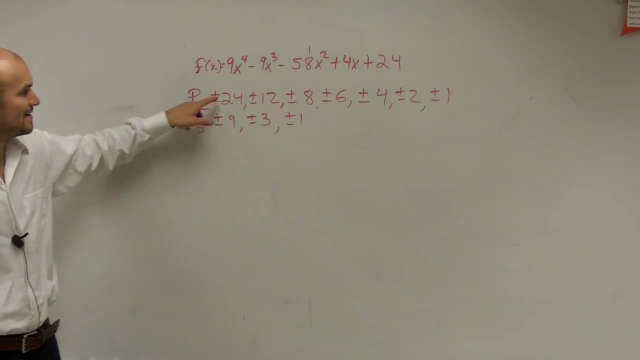 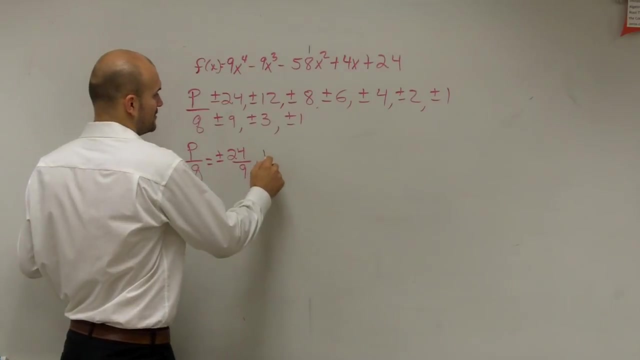 Right. So what I need to do is I need to put every single one of these numerators over each one of the denominators. This is a big problem, right? This is going to be a lot of solutions. So p over q is plus or minus 24 over 9, comma. 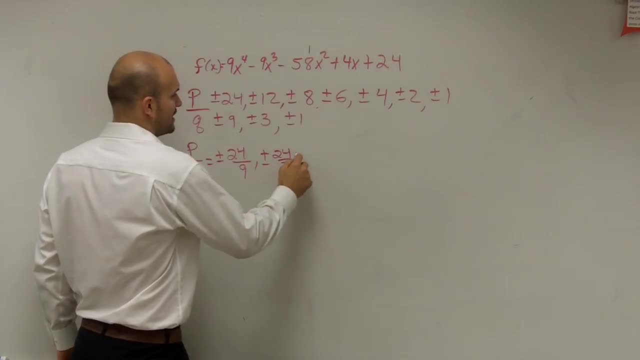 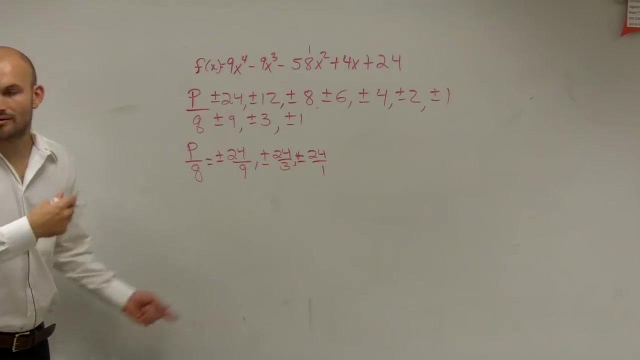 Plus or minus 24 over 3, comma. Plus or minus 24 over 1. right, right, I'm gonna, I'm gonna go and simplify them all. I'm just gonna write them all out and then you guys will see. oh, you don't need to write. 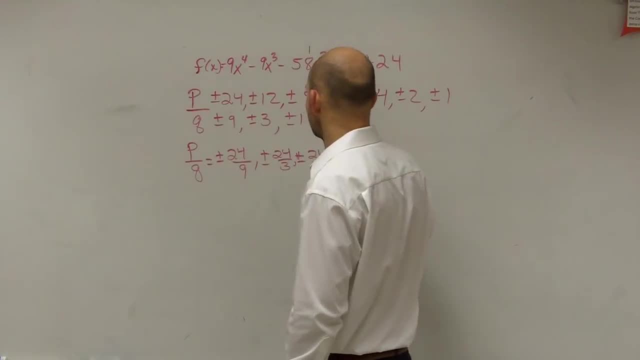 them all out. you can, can't, you know you can cut some out, if you don't. if once you see duplicates- because you don't need to write in duplicates- if you have extras, then you can eliminate them. so then I have plus or minus 12 over 9. 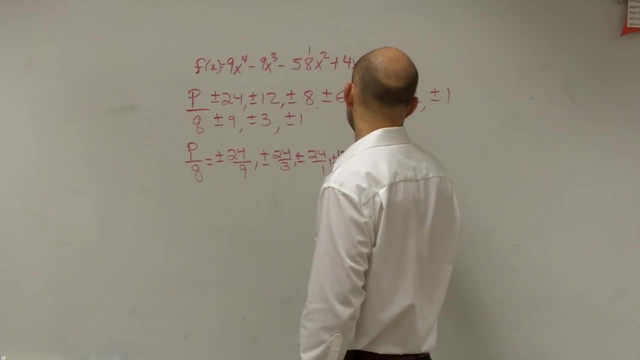 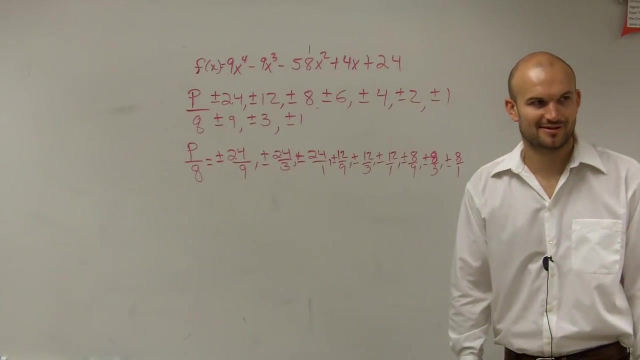 comma plus or minus 12 over 3 plus or minus 12 over 1 comma plus or minus 8 over 9 comma plus or minus 8, 8 over 3 comma plus or minus 8 over 1. that way kind of finally seeing my my trend that I'm doing here. this is a lot of problem. 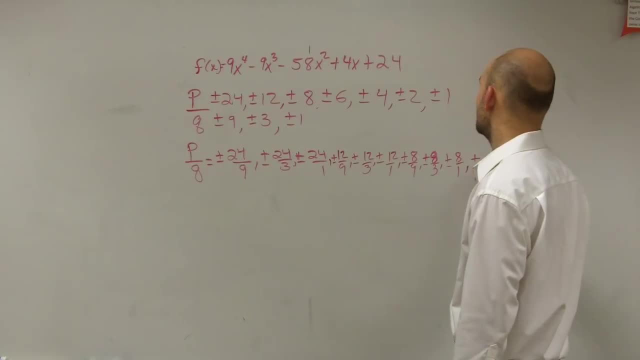 this is a lot of them, but we'll go through them. so we have comma plus or minus 6 over 9, comma plus or minus minus�� 0, 6 over 3, comma plus or minus 6 over 1.. I am running out of space so I'm going to continue over here. 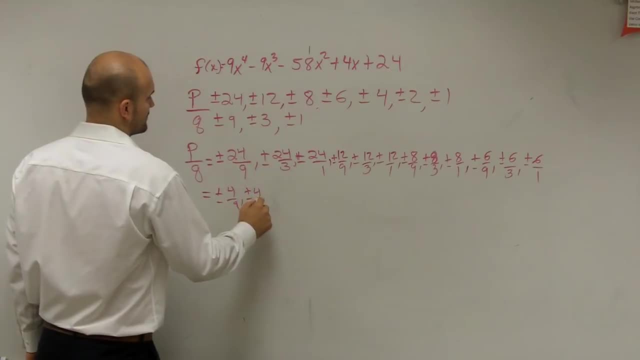 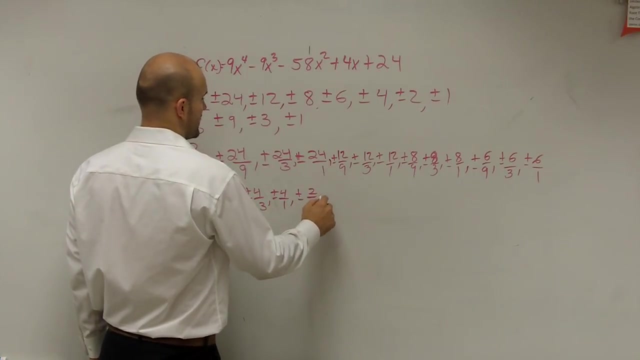 Comma: plus or minus 4 over 9, comma. plus or minus 4 over 3, comma. plus or minus 4 over 1, comma. plus or minus 2 over 9, comma. plus or minus 2 over 3, comma. plus or minus 2 over 1,. 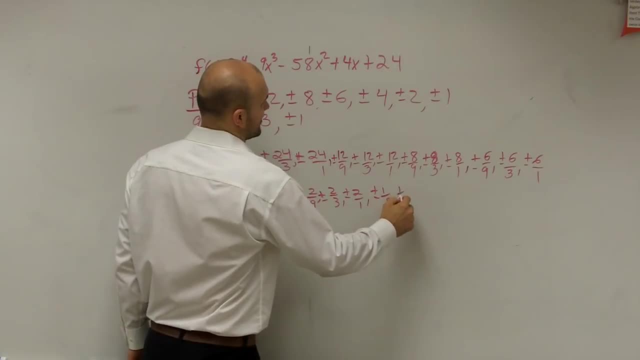 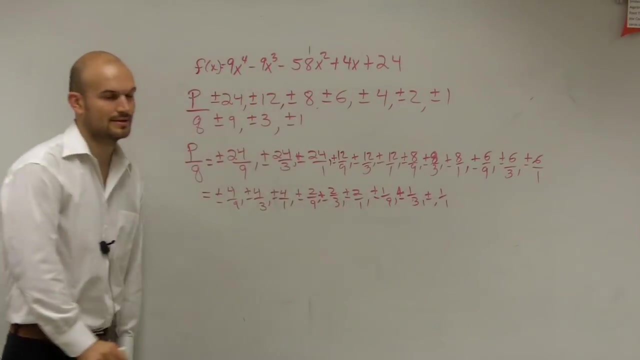 comma plus or minus 1 over 9 comma plus or minus 1 over 3 comma plus or minus 1 over 1.. All right, this one has a lot, and there's also some duplicates in here that we don't need to. 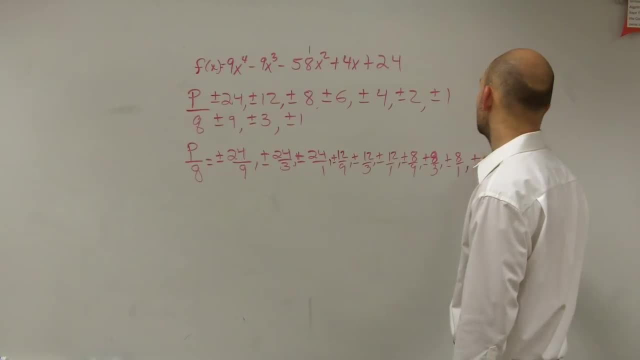 this is a lot of them, but we'll go through them. so we have comma plus or minus six over nine, comma plus or minus 6 over 3, comma plus or minus 6 over 1. I am running out of space so I'm going to. 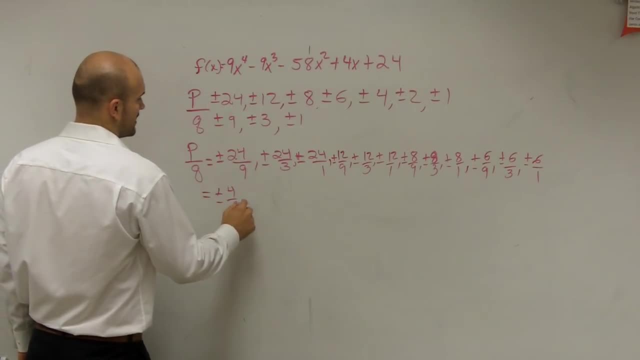 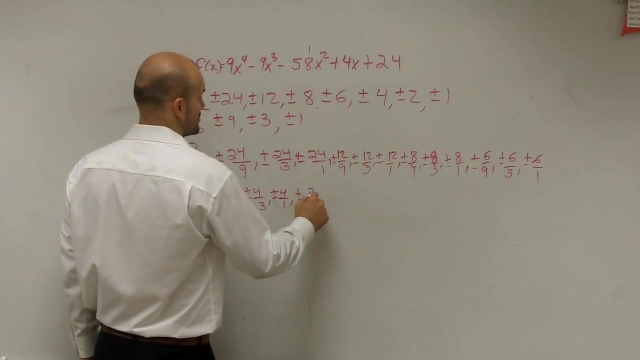 continue over here comma. plus or minus 4 over 9 comma. plus or minus 4 over 3 comma. plus or minus 4 over 1 comma. plus or minus 2 over 9 comma. plus or minus 2 over 3 comma. plus or minus 2 over 1 comma. plus or minus 1 over 9 comma. 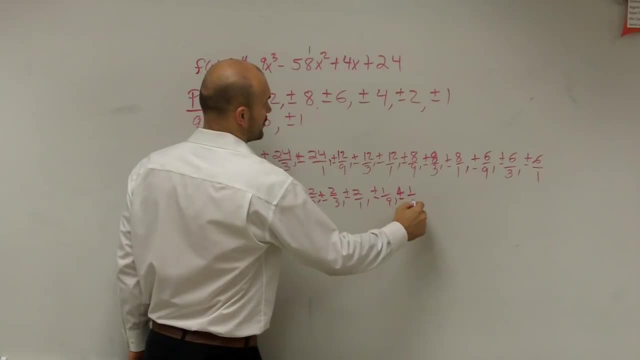 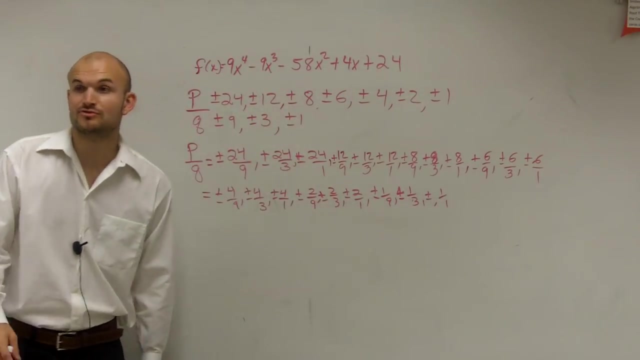 plus, plus or minus 1 over 3 comma. plus or minus 1 over 1. all right, this one has a lot, and there's also some duplicates in here that we don't need to keep on rewriting, right, we just all I need to. all I want you to do is just tell me the 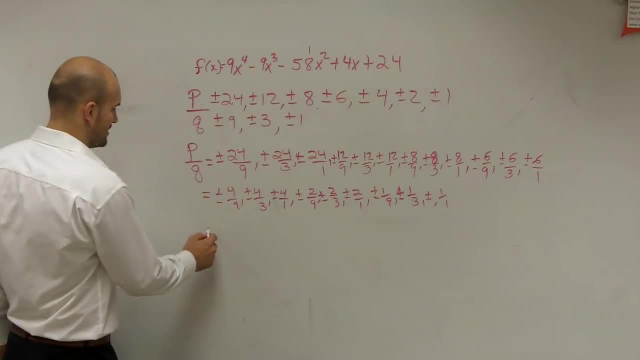 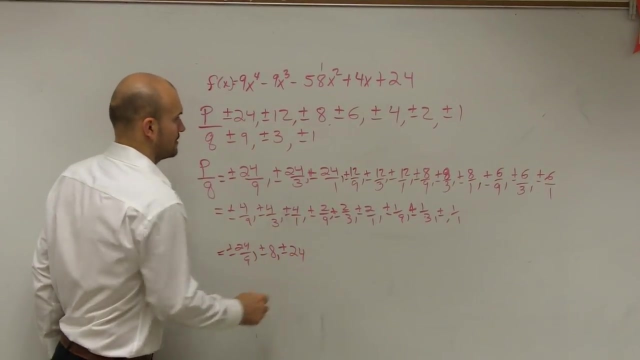 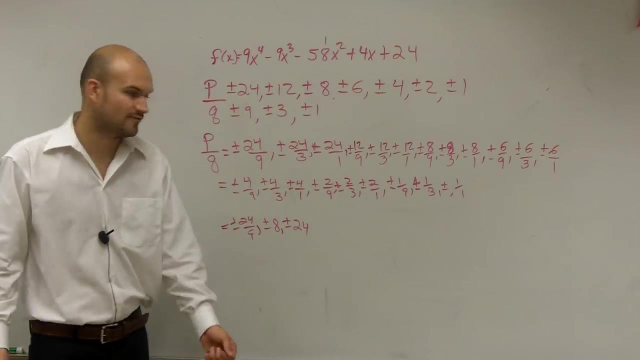 possible. so when you look at this, 24 or 9, that's going to be equals. plus or minus 24 over 9, 20, 24 over 3, that's really plus or minus 8. right then I have plus or minus 24, plus or minus 12 over 3. it can be we can reduce to 3 would be 4. 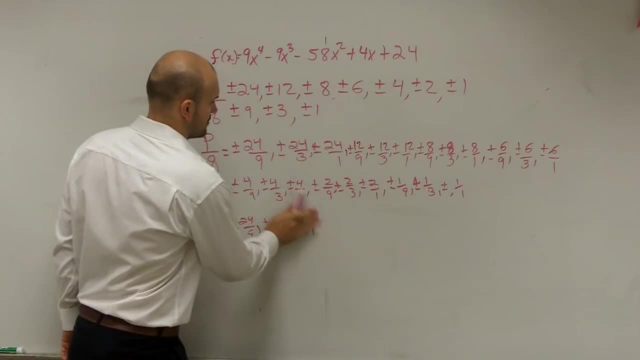 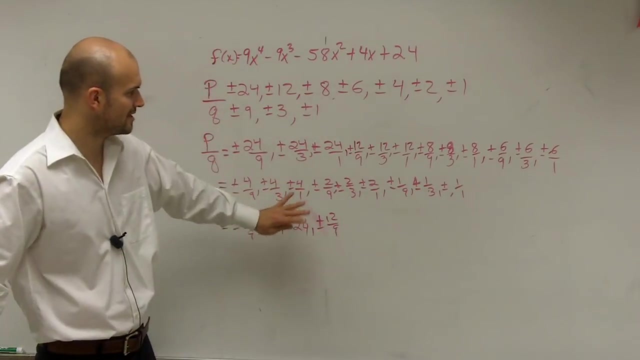 of thirds, 24 over 9, I could. I could go ahead and reduce it. you're right. I'll just actually I'm just gonna leave it right now as a 12 over 9. well, actually, we're just gonna never mind, we're just gonna leave it as however they are, 12 divided by 3, though we can. 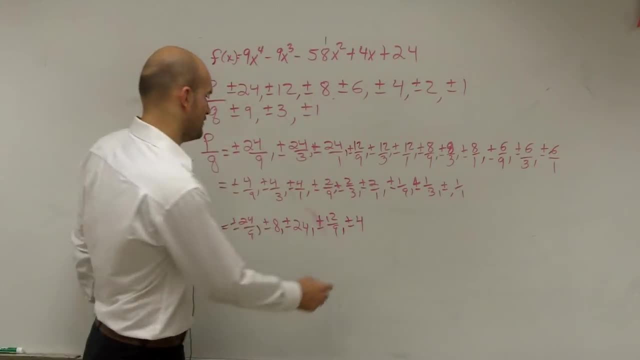 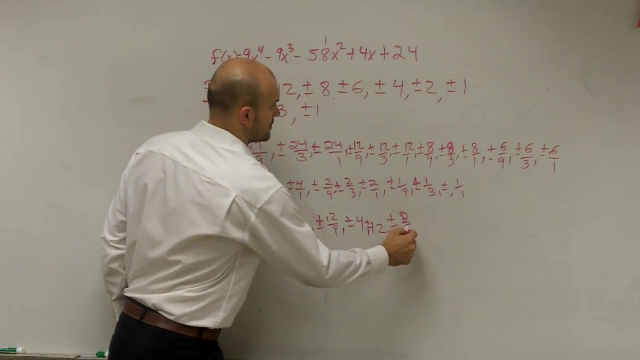 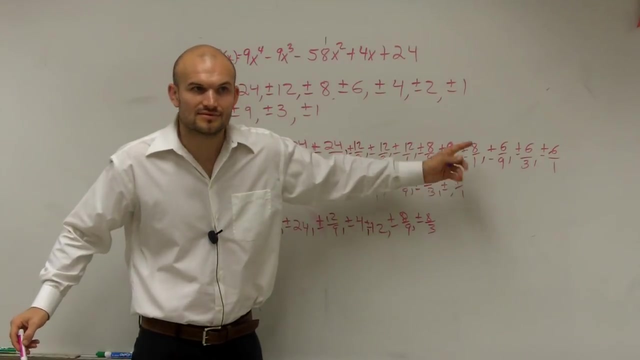 reduce to 4. 12 over 1 can be 12 plus or minus. these are all plus or minus. let's 8 over 9, 8 over 3. however, you guys can see, I already have 8 right, so I don't. 8 over 9. 8 over 3. however, you guys can see, I already have 8 right, so I don't. 8 over 9, 8 over 3. however, you guys can see I already have 8 right, so I don't need to continue that 6 over 9 is going to be 2. need to continue that 6 over 9 is going to be 2. 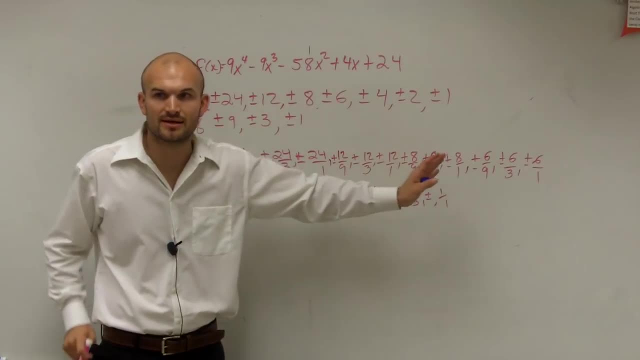 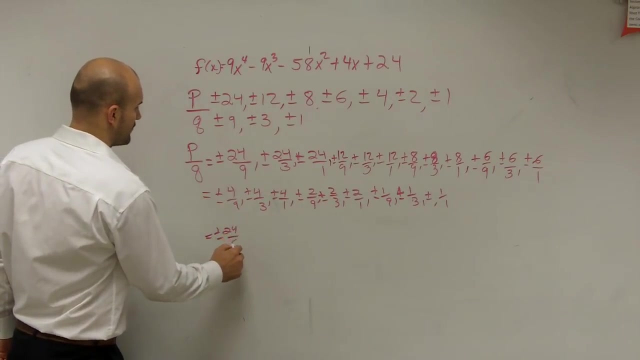 keep on rewriting, right? All I want you to do is just tell me the possible. So when you look at this, 24 over 9, that's going to be equals plus or minus 24 over 9.. 24 over 3, that's really plus. 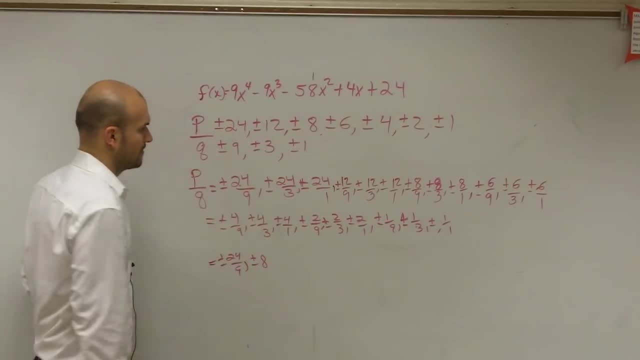 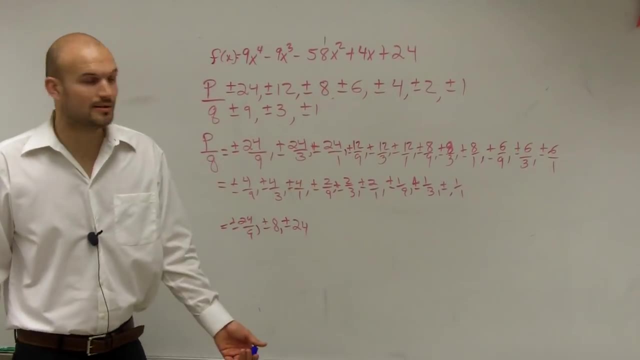 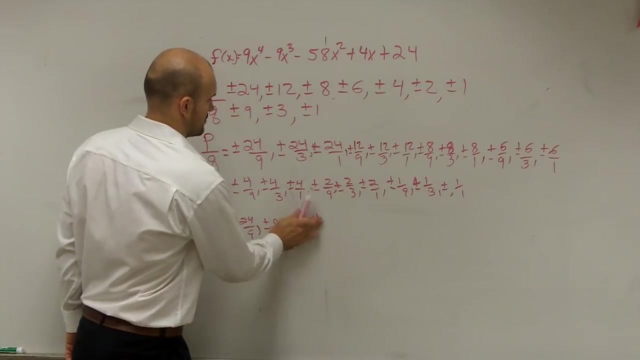 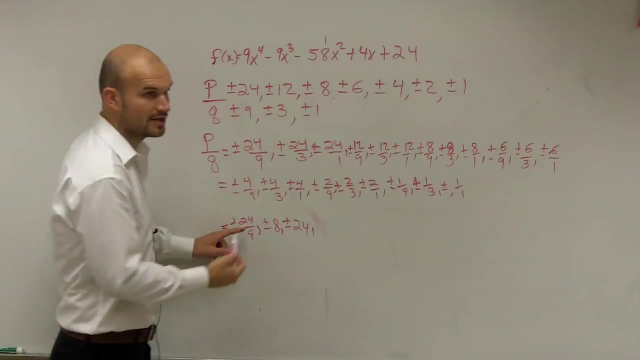 or minus 8, right, Then I have plus or minus 24, plus or minus 12 over 3.. It can be, we can reduce to 3, it would be 4 thirds 24 over 9, I could, I could go ahead and reduce it, you're right. 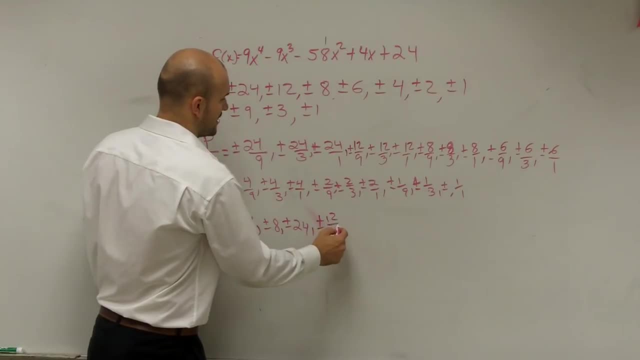 I'll just- actually I'm just going to leave it right now as 24 over 9.. 12 over 9.. Well, actually, we're just going to never mind. we're just going to leave it as, however, they are 12 divided by 3, though we can reduce to 4.. 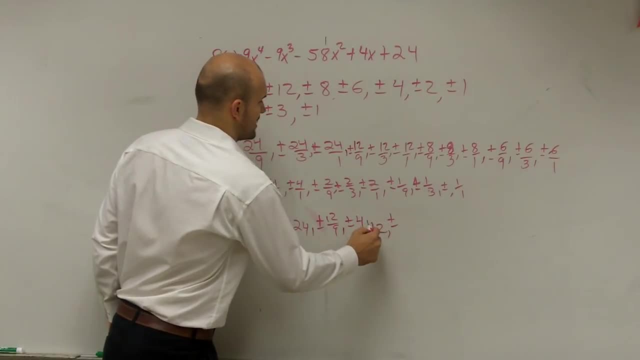 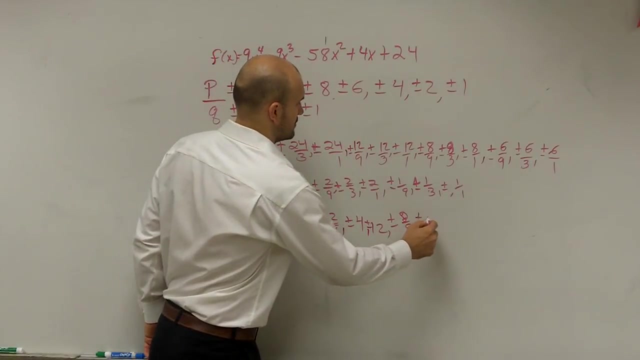 12 over 1 can be 12.. Plus or minus. these are all plus or minus. That's 8 over 9.. 8 over 3.. However, you guys can see I already have 8, right, So I don't need to continue that. 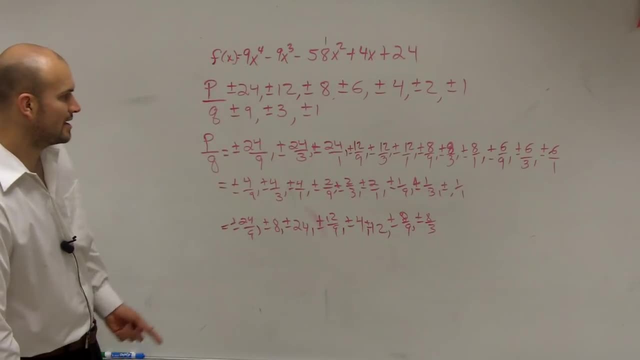 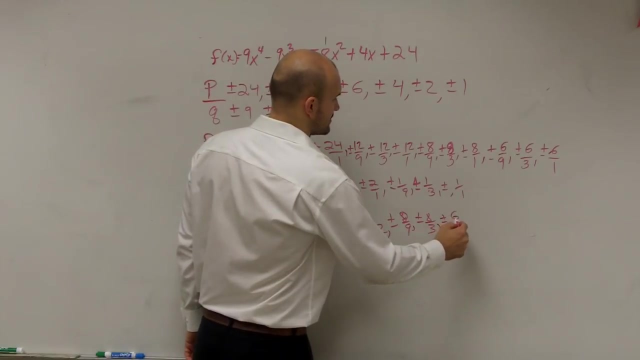 6 over 9 is going to be 2 thirds, and do I? I don't have a 6 over 9.. Plus or minus 6 over 9, 2 thirds, plus or minus 2,, which I do not have yet, right. 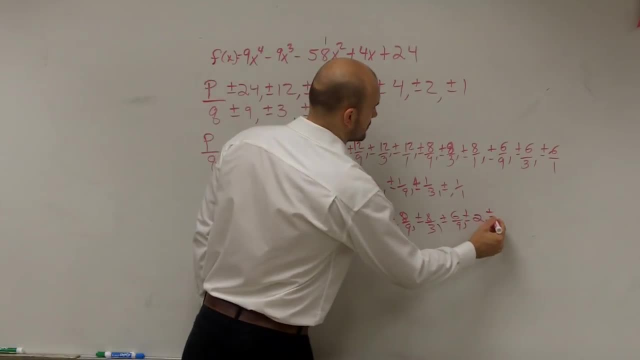 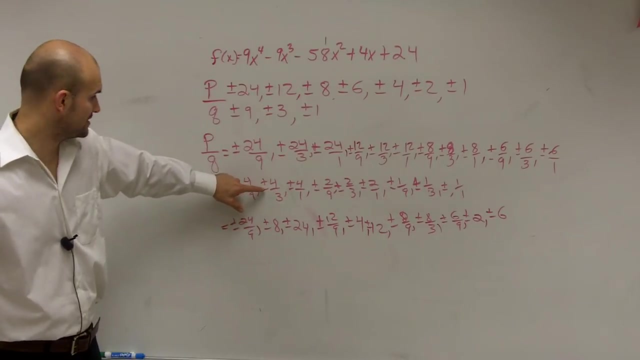 2, and do I have a 6?? Nope, Let me look over here. I have 4 ninths Now actually. you can see here: yeah, when I reduce this right, that's, that is 4 thirds, right, So I can reduce that down to 4 thirds and you can see. 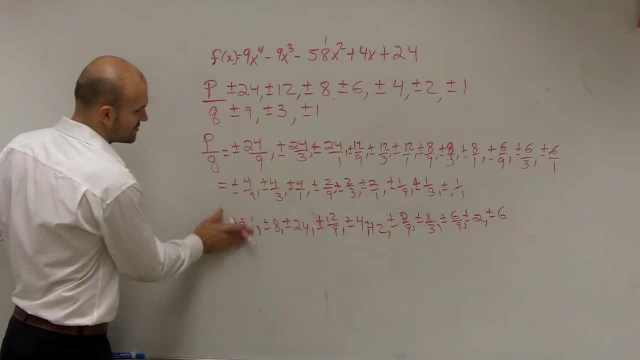 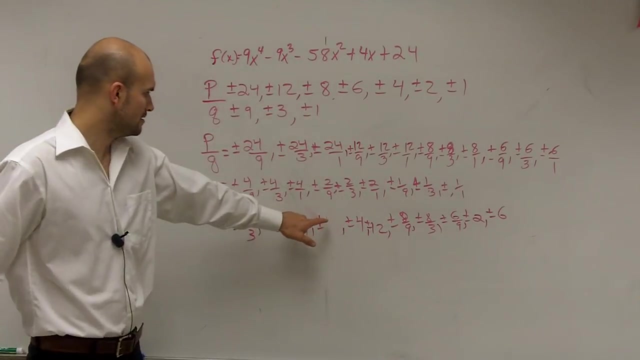 that these are the 6 thirds. So I can reduce that down to 4 thirds and you can see that these are the same. So I don't need to include this other 4 thirds, because this actually is reduced down to 4 thirds. Actually, I mean, let's write that down as that one is hold on. that was the same thing. 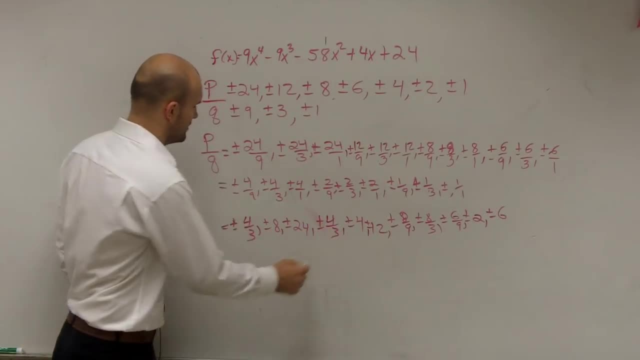 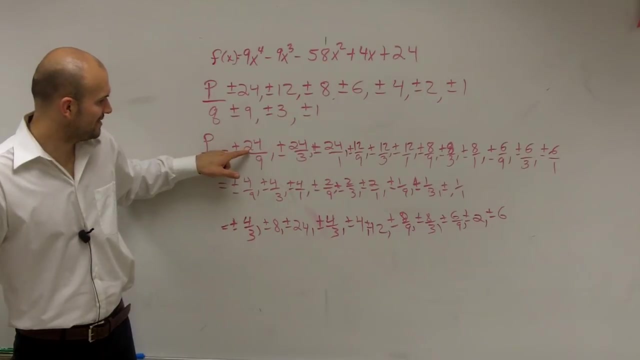 wasn't it? Yeah, Sorry, you can't see it. 24 over 9 is the same thing, or no? that was. that's. 6 divided by 3 is going to be 8.. That's 8 thirds, not 4 thirds. This one is 4 thirds. 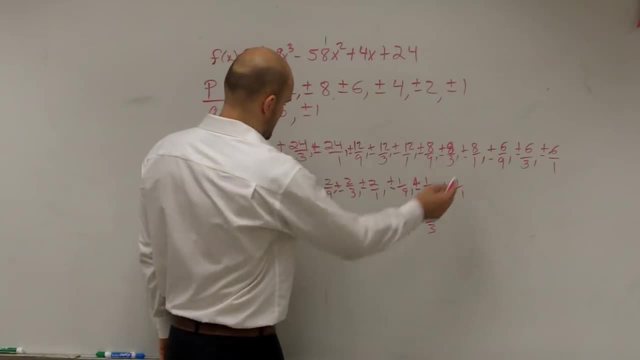 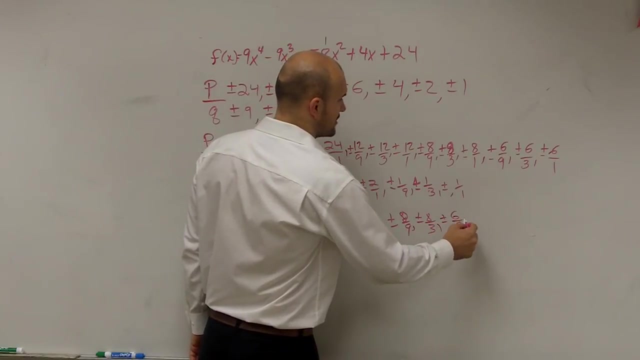 need to continue that 6 over 9 is going to be 2 thirds. and do I? I don't have a 6 over thirds. and do I? I don't have a 6 over thirds. and do I? I don't have a 6 over 9, plus or minus. 6 over 9, 2 thirds plus or. 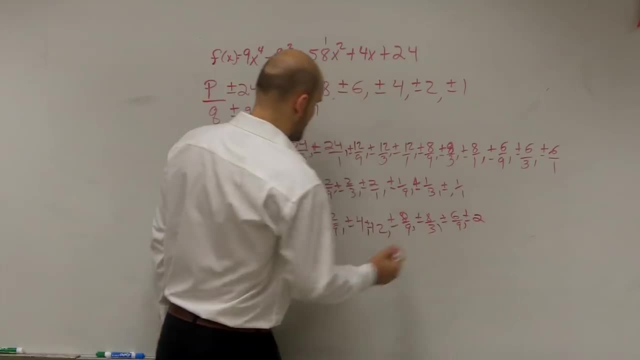 9 plus or minus 6, over 9, 2 thirds plus or minus 2, which I do not have yet right. 9 plus or minus 6, over 9, 2 thirds plus or minus 2, which I do not have yet right. 9 plus or minus 6, over 9, 2 thirds plus or minus 2, which I do not have yet right. 2 and do I have a 6? nope, let me look. 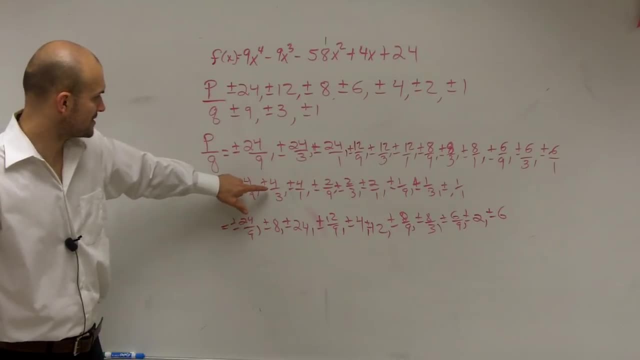 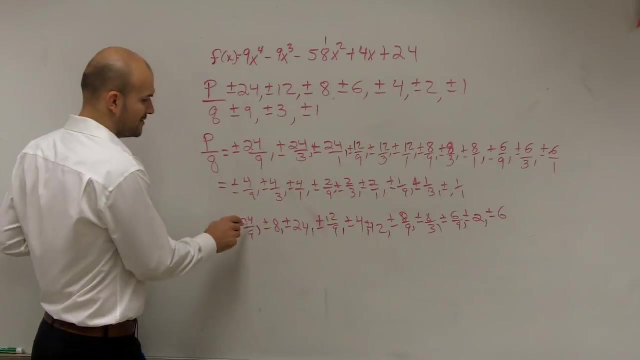 over here. I have four nights now. actually, you can see here, yeah, when I reduce this, right, that's that is four thirds, right, so I can reduce that down to four thirds and you can see that these are the same. so I don't need to include this other four thirds, because this actually is reduced down to four. 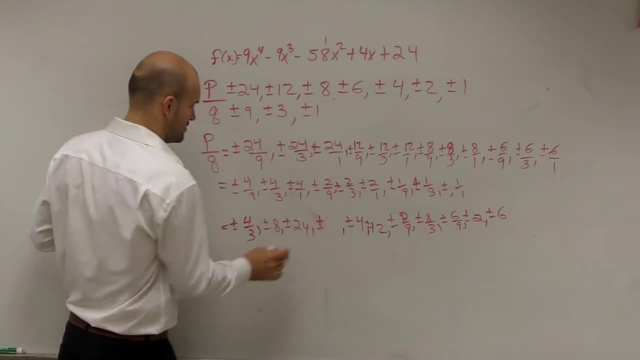 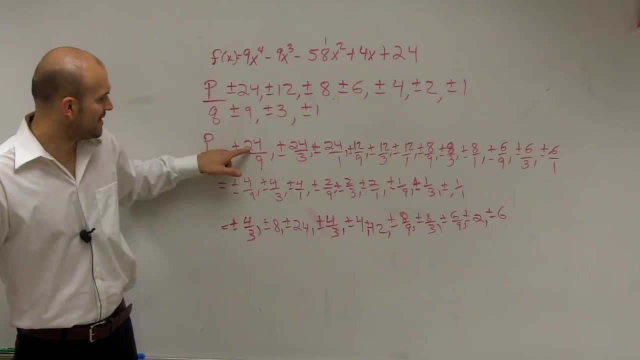 thirds actually? I mean which? let's write that down, as that one is. hold on, that was the same thing, wasn't it? yeah, sorry, you can't see it. 24 over 9 is the same thing, or no? that was that's. 6 divided by 3 is going to be 8. that's 8 thirds, not. 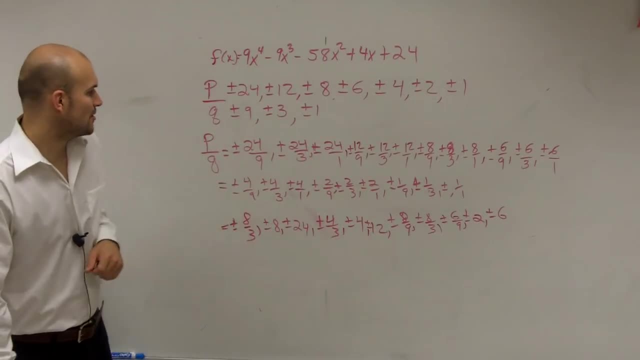 4 thirds. this one is 4 thirds, so what we see is here: I already have a 4 thirds when I reduce it, so I don't need to write that one. I already have a 4, so I don't need to write that. do I already have a 2 nights, you know? so I could do. 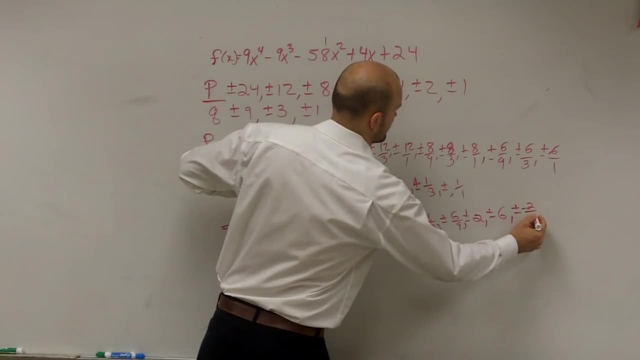 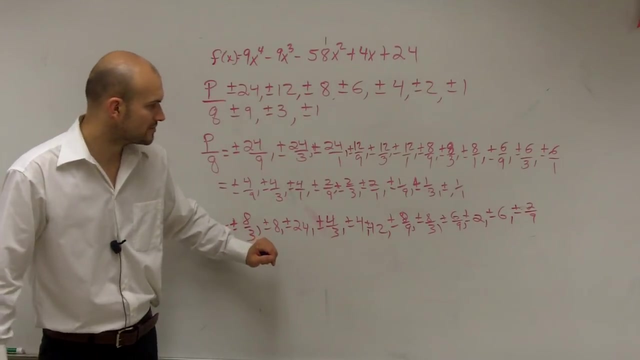 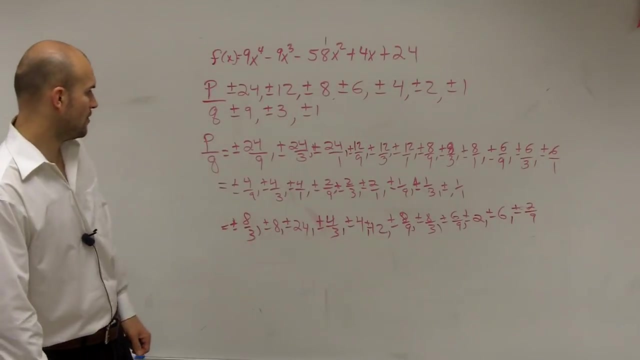 plus or minus 2 nights. okay, do I already have a 2 thirds? yeah, I already have a 2 thirds, which was right there that can reduce down to 2 thirds. I already have a 2. I do not have a 1 9th a. 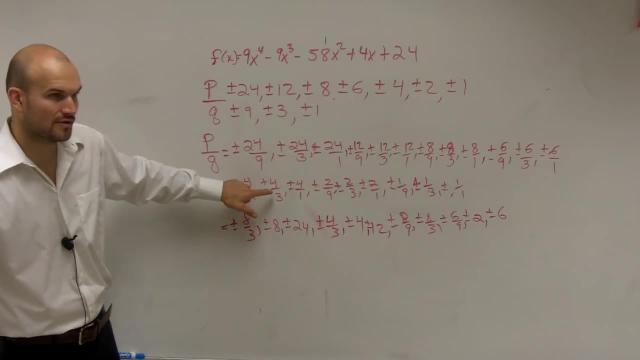 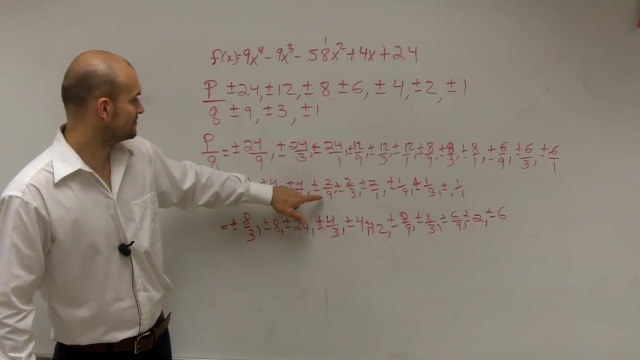 So what we see is here: I already have a 4 thirds when I reduce it, so I don't need to write that one. I already have a 4,, so I don't need to write that. Do I already have a 2 ninths? No, so I could. 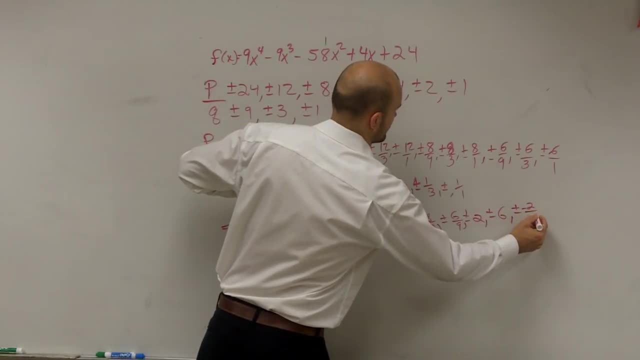 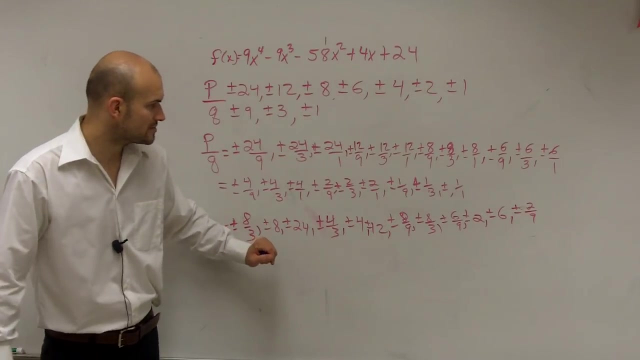 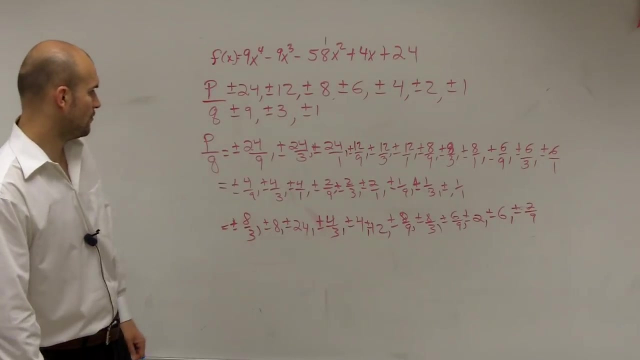 do plus or minus 2 ninths. Okay, do I already have a 2 thirds? Yep, I already have a 2 thirds, which was right there. That can reduce down to 2 thirds. I already have a 2.. I do not have a. 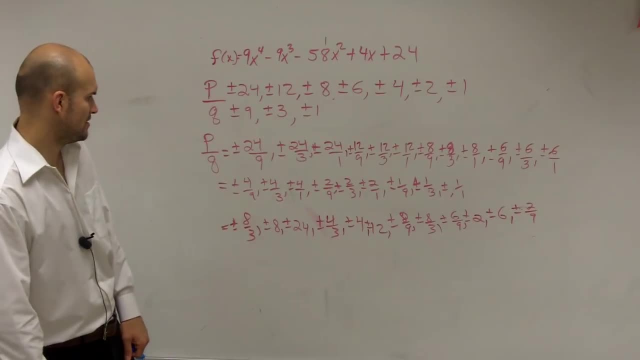 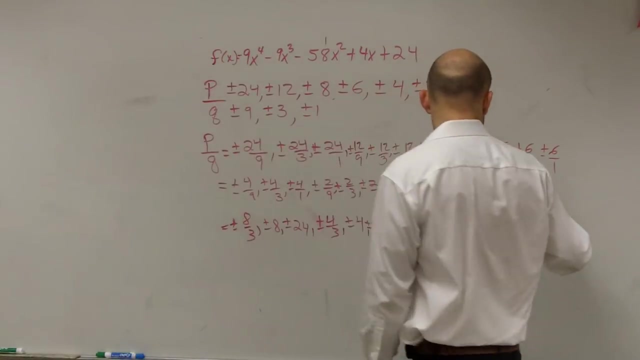 1 ninth, a 1 third, but I already have a 1.. No, I don't have a 1.. I don't have a. yeah, I guess it is my only 1.. So I don't have plus or minus. so I have 2 ninths, I already have 2 thirds, I already. 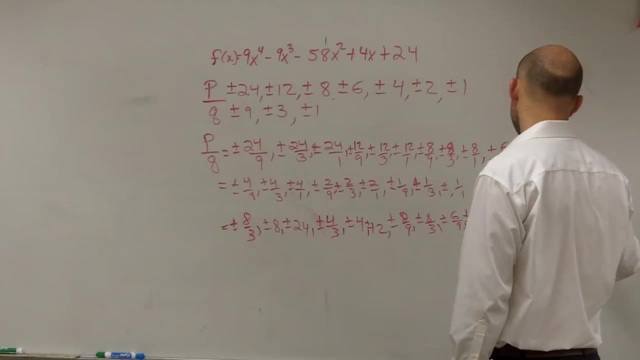 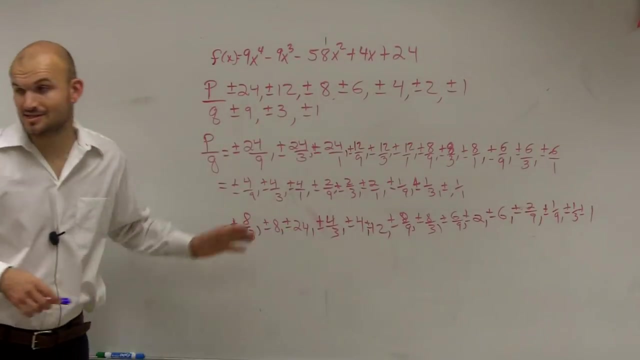 have 2, but I do not have a plus or minus 1 ninth comma. plus or minus 1 third and plus or minus 1.. It's a lot. This is probably going to be longer than anything else you even get on your test. but 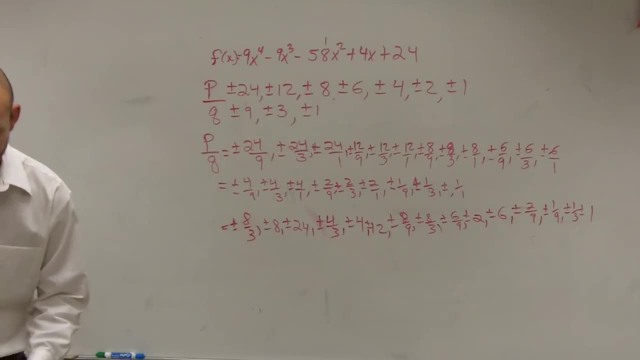 make sure you write down all the factors. all right, I'm going to leave it at that and then I'll go through finish the rest of the problem. So that's just doing your rational zero test. 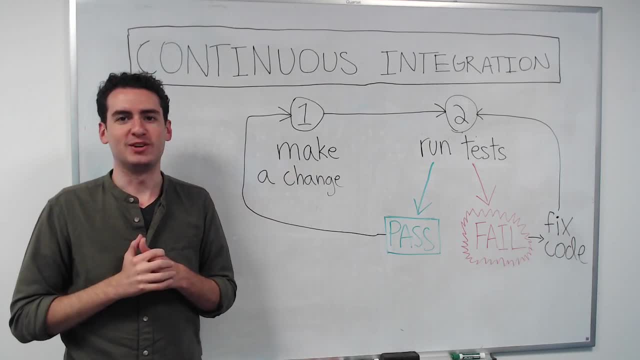 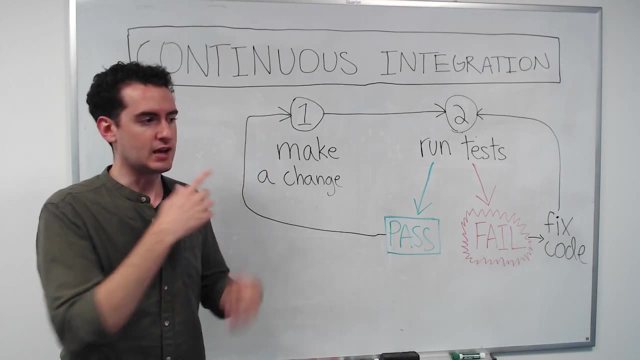 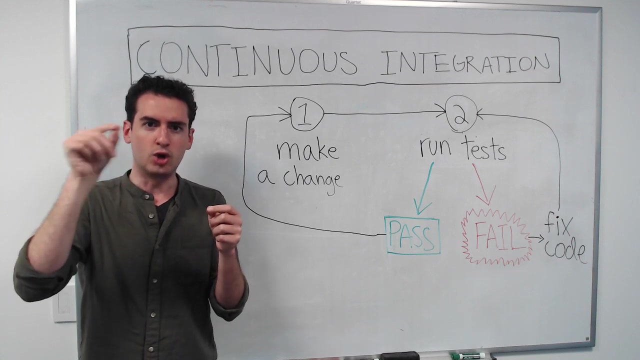 Hi folks, my name is Alec Sharma, I'm a developer advocate at CircleCI and I am here today to talk to you about continuous integration, which is a software development practice where everyone on the engineering team is continuously integrating these small code changes back into the code base. 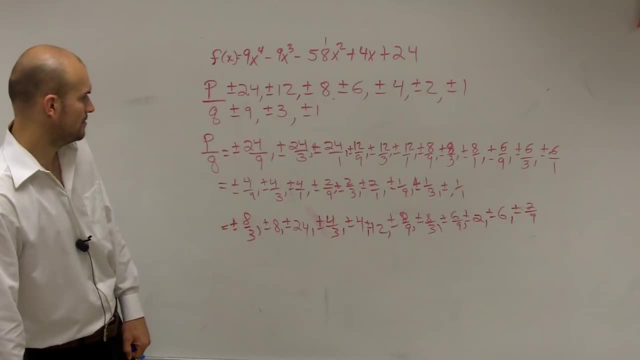 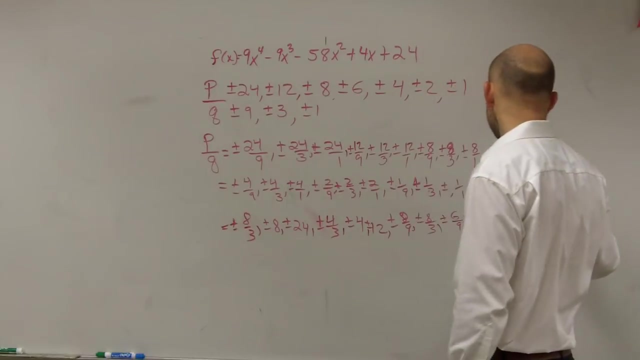 1. 3rd, but I already have a 1. no, I don't have a 1, so I don't have plus or minus 2. plus or minus 2 9ths, so I don't have plus or minus 2 9ths, so I don't have. 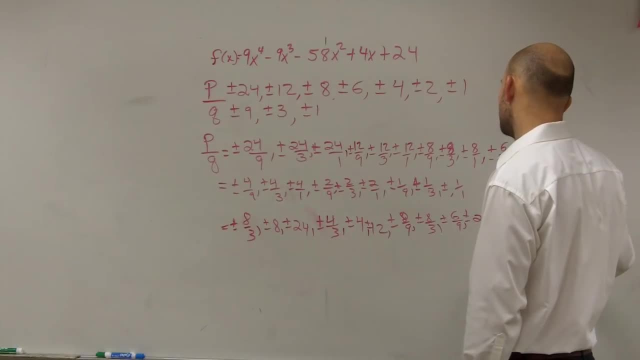 plus or minus 2 9ths. so I have 2 nights already have 2 thirds, already have 2, but I do not have a plus or minus 1 9th comma. plus or minus 1 3rd and plus or minus 1. it's a lot. this is probably going to be longer than anything else.